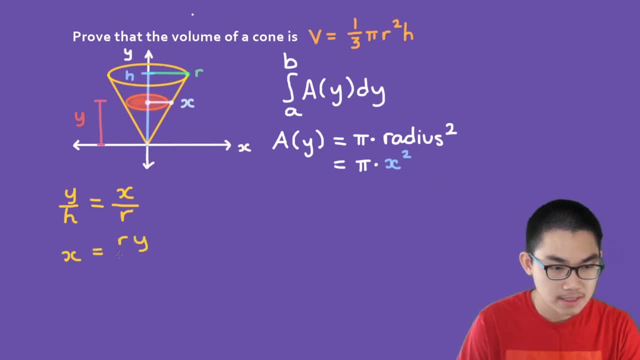 be r times y divided by h. So if we rewrite this, the area will be pi times the radius times y divided by h, to the power of 2.. Which will simply be pi times the radius squared divided by the height squared times y squared, And we can also rewrite this one more. 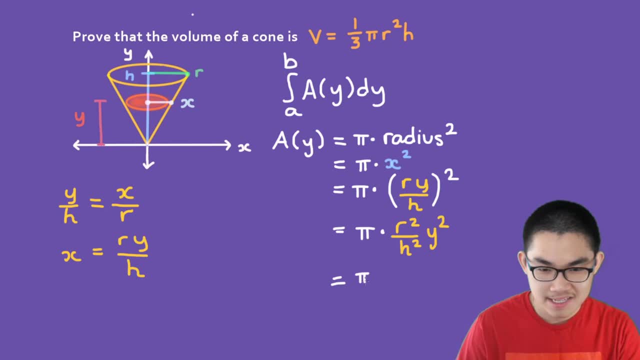 time to make it even simpler, as pi times the radius squared divided by the height squared squared divided by the height square times y square. and so we successfully found the formula for the area of this cross-section and we are ready to substitute into our integral. so now we 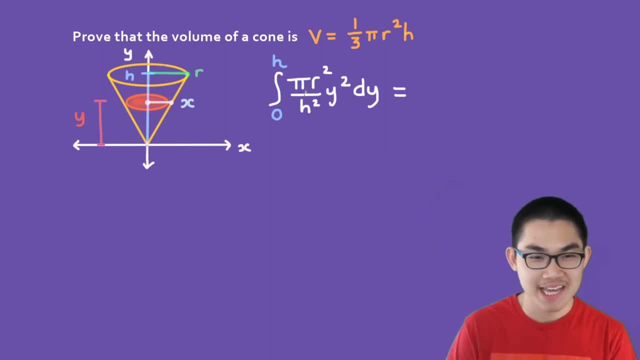 replace the ay with our area formula and the volume of this integral is from zero to h. that is going to be this zero to this h of pi times the radius squared divided by the height, square times y square. since pi and the radius and the height are just constants, we can move them. 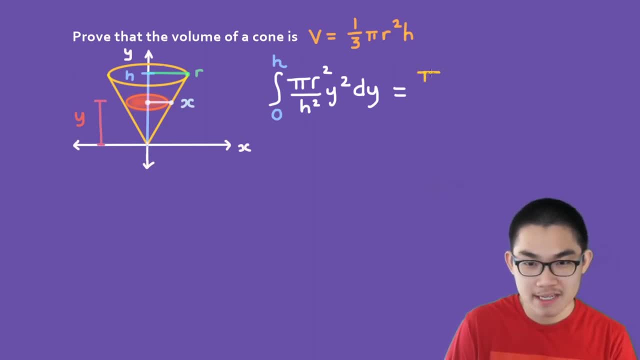 outside of the integral. so this will simply be pi times the radius squared divided by the height square times the integral from zero to h, of y to the power of two. and this integral is actually very easy to solve: this is just pi times the radius squared divided by the. 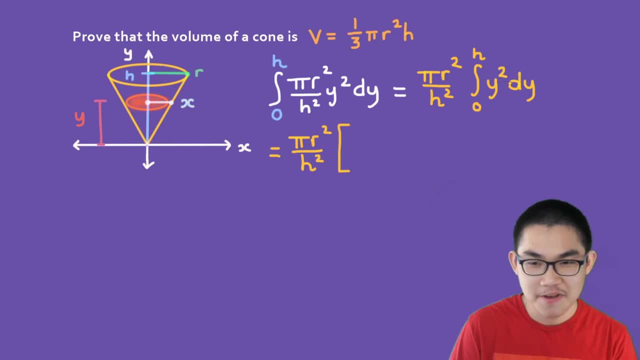 height square times the anti-derivative of y to the power of two. and so remember the anti-derivative. you just take the two, you plus one, so let's do that. first that's going to be y to the power of three, and then you divide by that exponent, so that's going to be one over three, and don't. 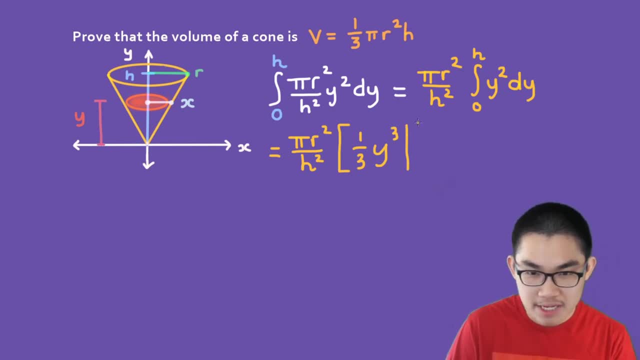 forget the upper and the lower bound, which are h and zero. again, this is just going to be pi times the radius squared divided by the height square. now we have to substitute the h and the zero into this formula, so it's going to be one over three times the height to the power of three, so the height to